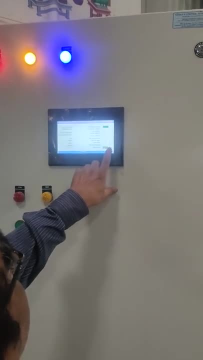 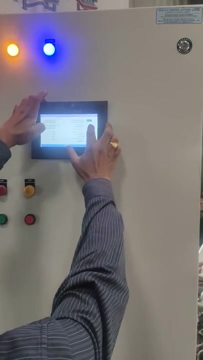 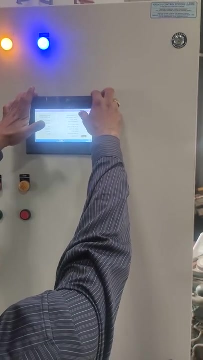 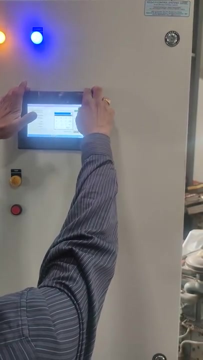 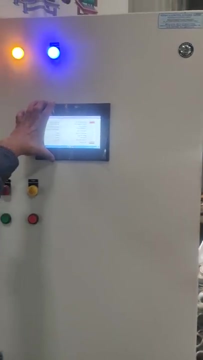 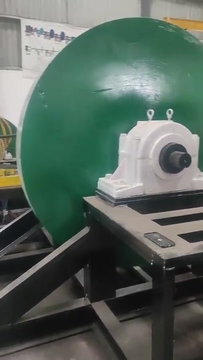 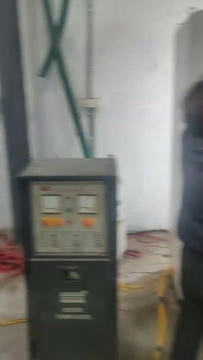 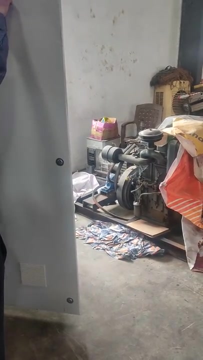 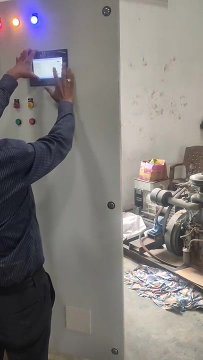 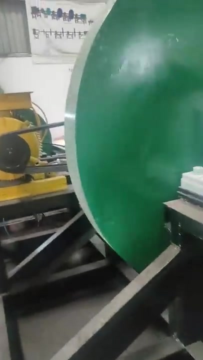 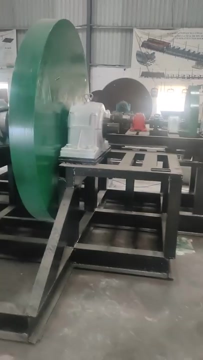 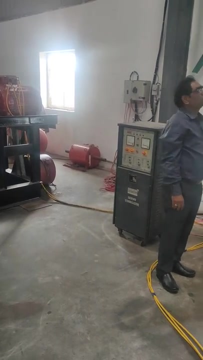 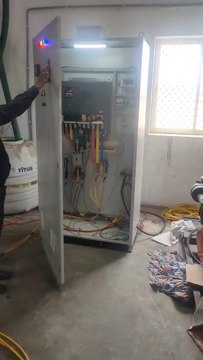 Ok, So here this is stop and it will start rotating. Ok, In the start. Yes, So this is started Slowly. we are increasing the speed, sir. Ok, We have started it slowly. It is in a slow start. It will go up very slowly: First 50, then 50, then 100.. In this way, we will be taking the thing into consideration, Ok. 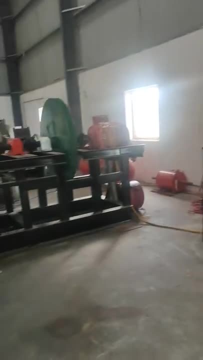 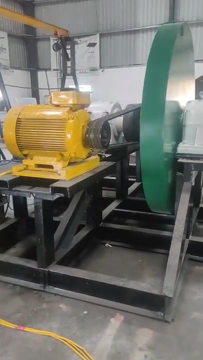 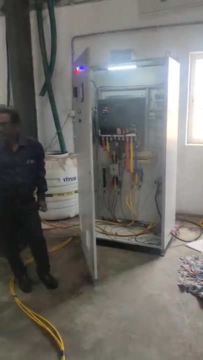 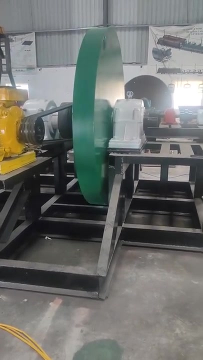 Ok, Now it is moving. Now it is moving slowly, So once we cross 50, we can take that to 100.. Now it is 100.. Ok, Now it has given a command above 100.. Ok, So it will start moving. 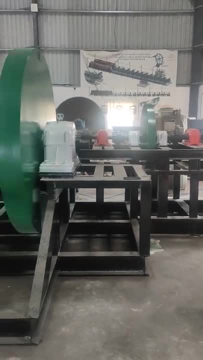 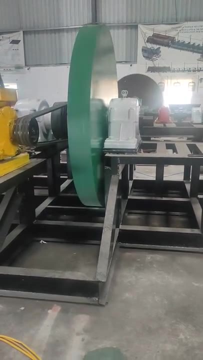 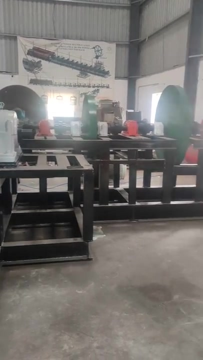 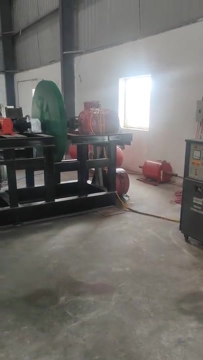 150.. Now it has given a command of 150.. This is a unique thing. No scientist has done this in the world, Isn't it? Yes, Now it has come to 200.. It has given a command of 200.. 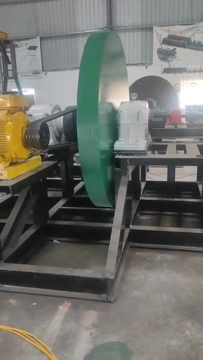 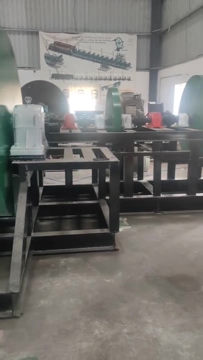 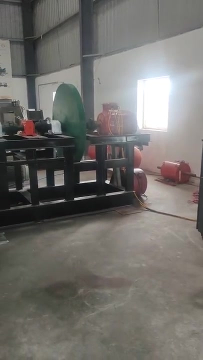 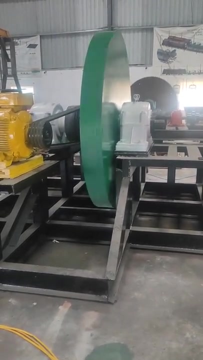 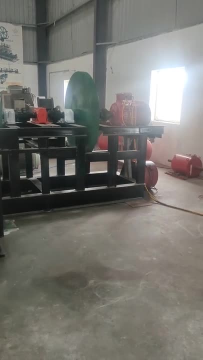 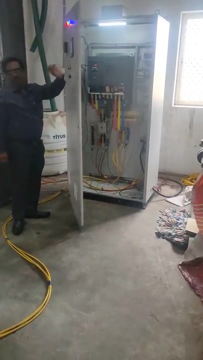 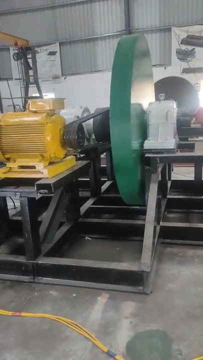 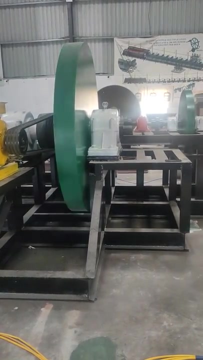 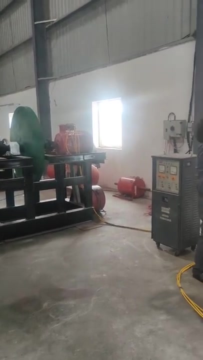 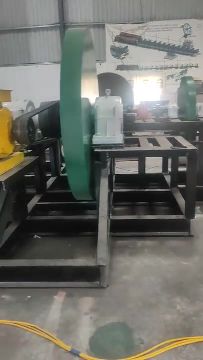 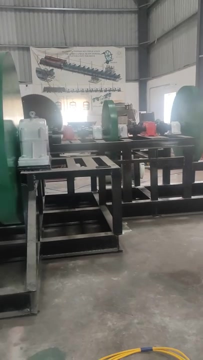 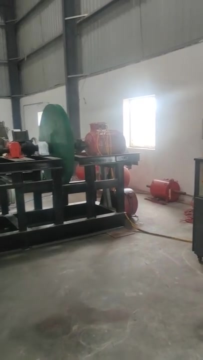 There is no such person in India who has done such a thing. No one has done it outside. They have put it on 300.. They have put it on 350.. It has come on 350.. Total will go on 450.. 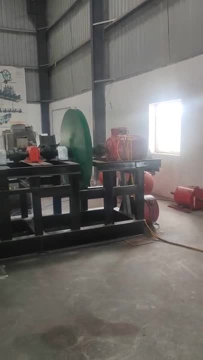 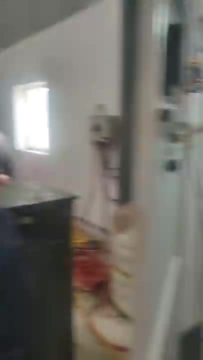 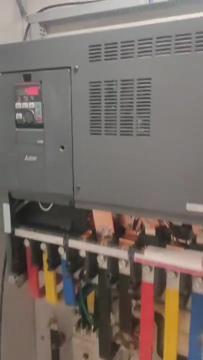 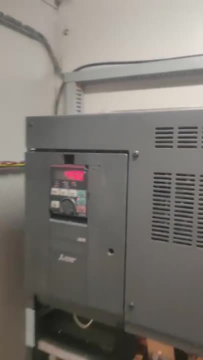 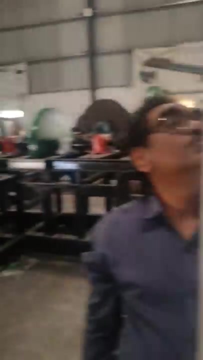 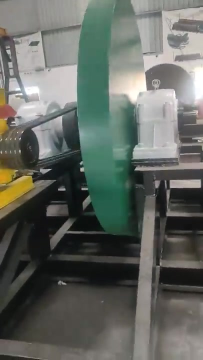 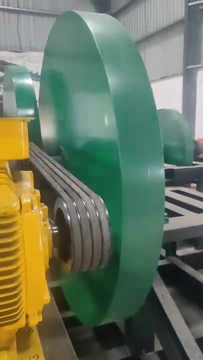 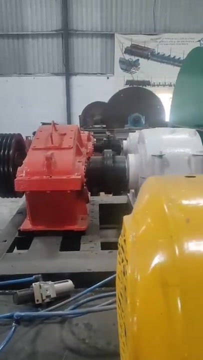 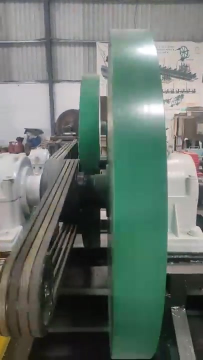 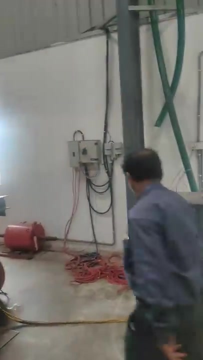 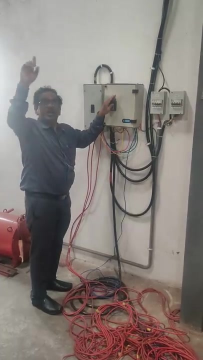 Now, it has come on 450.. Ok, It has come on 450.. Ok, It has come on 450.. Ok, It has come on 450.. Yes, Now we will take the load. Did it turn on? Did it turn on? 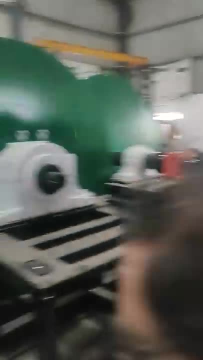 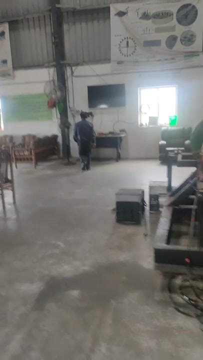 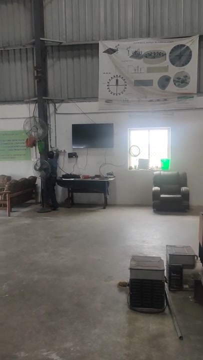 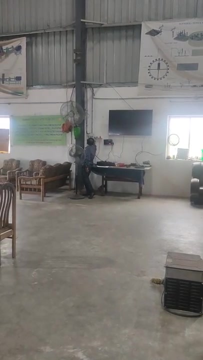 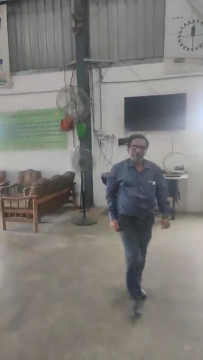 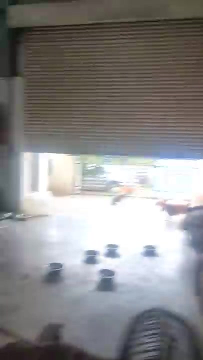 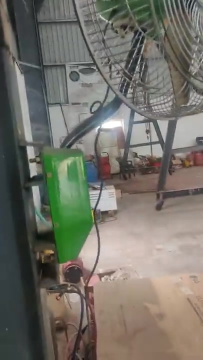 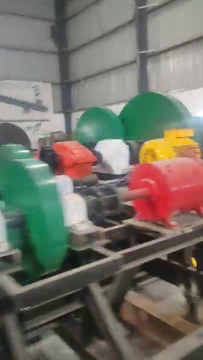 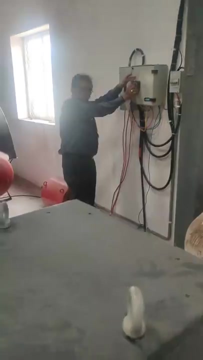 No, the lights, The lights, The lights. Yeah, we have to on the lights. we have to on the load. everything, fan, fan, fan. yes, we have to switch on the load. yes, we have the load. yes, we have the load. now i should switch on. yes, we have to switch. 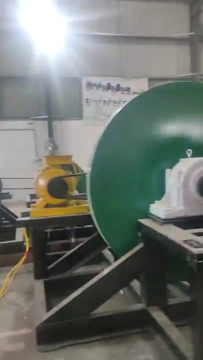 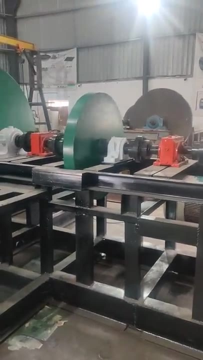 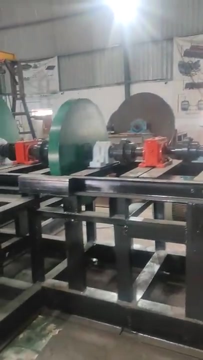 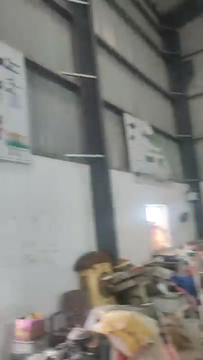 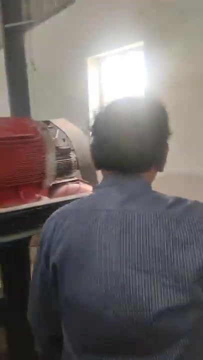 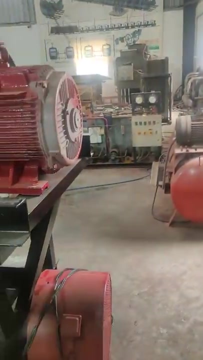 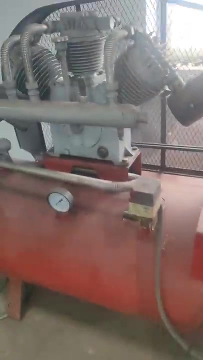 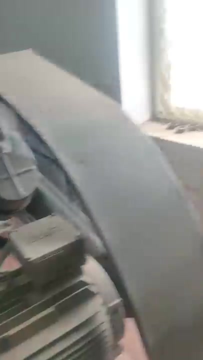 on. yes, So this is running on the generator. okay, So everything is running on the thing. So this is running on the thing. so this is then. we know it's a compressor. Compressor is also running. okay, this compressor is also running, okay. okay, compressor is. 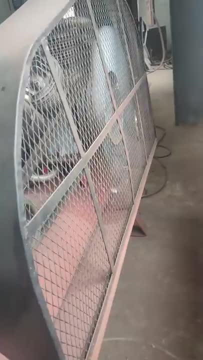 also running, completely Okay. So this is how everything is running. You can leave it like this, no matter how long it runs, it's up to you. This will continue to work for as long as it will. okay, There is no stoppage for this. 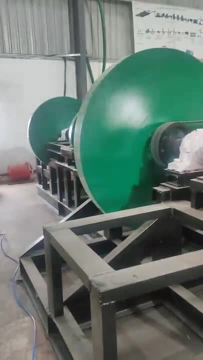 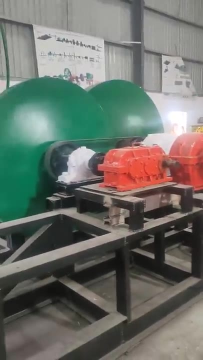 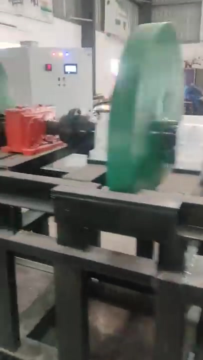 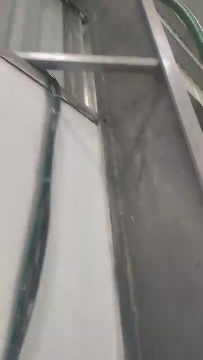 Ok, Yes, No one has done this till today. If you put the load, it stops. But see, this Compressor is put And whatever lighting is there, Whatever it is All together, We put the light here too. Put this light too. Ok, This light is also on Now. the entire workshop. 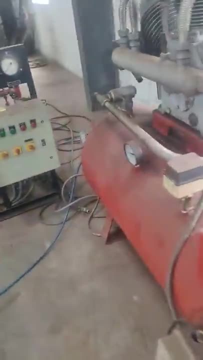 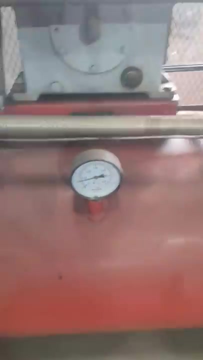 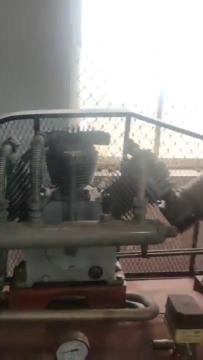 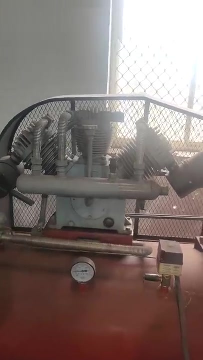 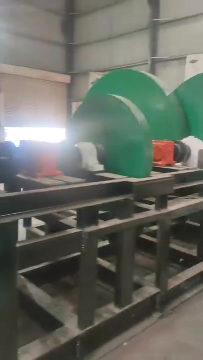 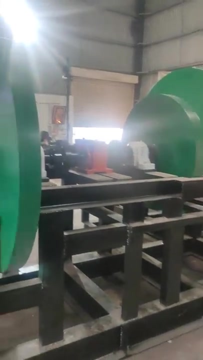 This is all running, Ok, And this is. This is also working. Ok, This is also. This is your 10 kilowatt, This is, And All these things are running. Ok, Everything is perfect In the system. Flywheel- Everything is on. The system is running. If I All these things, 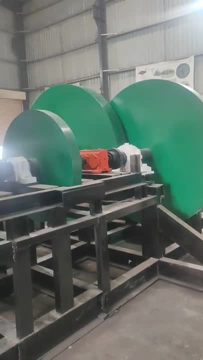 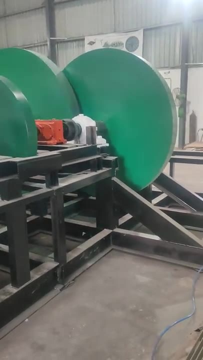 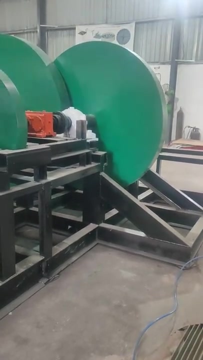 Take out and do the same flywheel And do this 4 meter So it becomes even easier for me. This is 12 tons. If I give 12 tons As the same flywheel, Then my more Energy is generated. 46 kilowatt is generated In 4 meter. 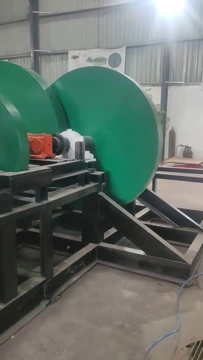 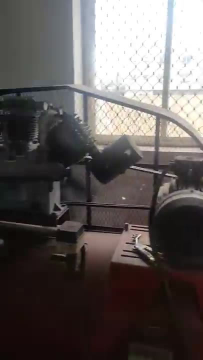 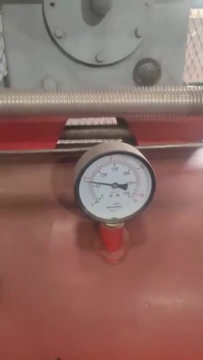 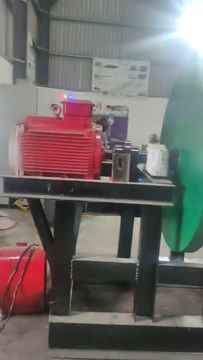 According to this system, 46 kilowatt is generated. So you have to see this very well. See, this is running Ok In this way. How much time you take, How much time you take, 24 to 7, 365 days, There is no problem, Ok, Ok. 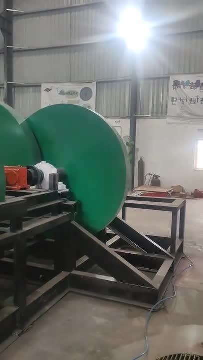 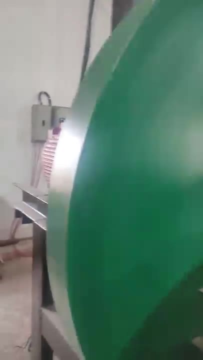 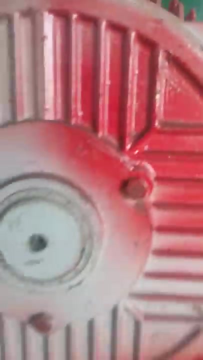 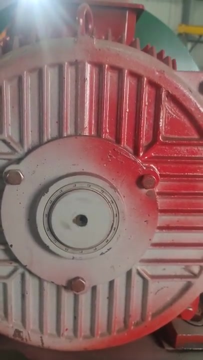 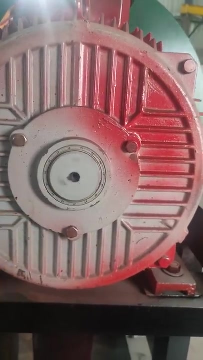 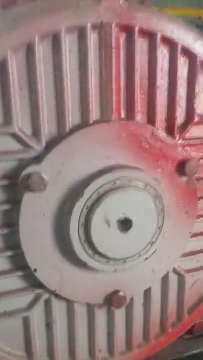 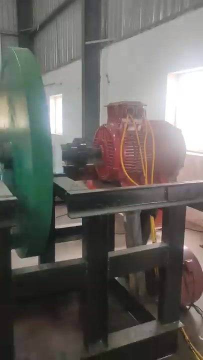 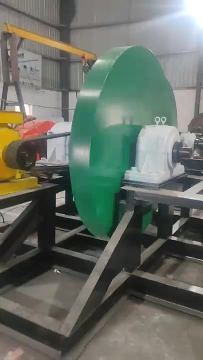 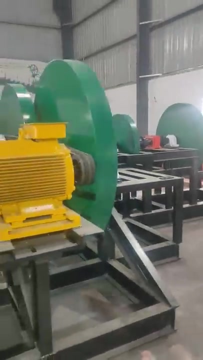 Ok, Let me show you Here This is 4 meter ferris wheel, And here Here This is, And by this It is running at maximum 40 to 50 rpm. it is not running much, so in this way it is going to run completely. so this is the energy generated by your flywheel, so in this energy you can show your superior strength. and this technology is not anywhere. 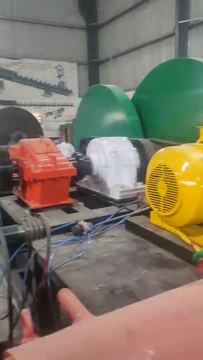 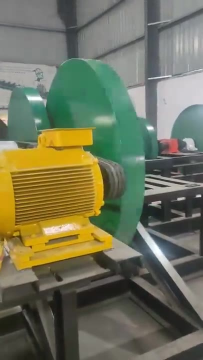 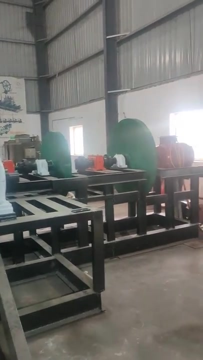 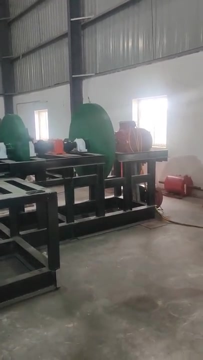 It is not anywhere in any country. okay, with this technology we can generate anywhere. multi megawatt diameter. rpm weight is the core raw material for this technology. gamma gear, private limited gamma gear. flywheel kinetics. associated mass mechanical applications is the principle of gamma gear kinetics. associated mass mechanical applications is the principle of gamma gear. 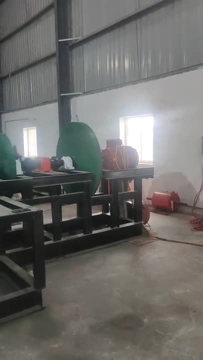 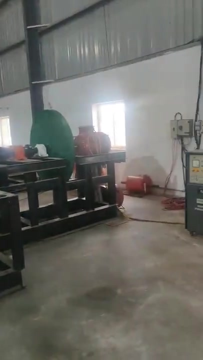 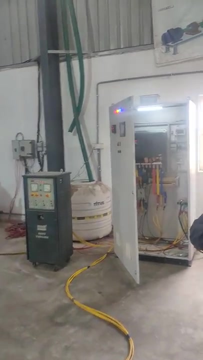 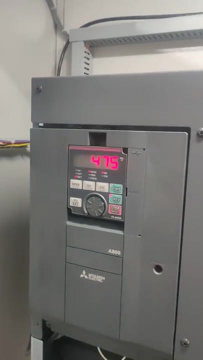 But the mechanical power to get extracted from the flywheel- see, it is getting extracted. no matter how many times, no matter how long, no matter how much time you do it, it will keep running. there is no problem in it. and this is see, it is up to 475, we have taken its rpm to 475, okay. 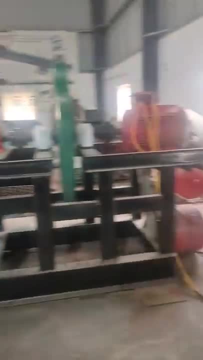 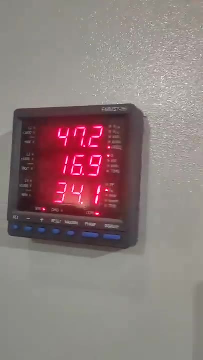 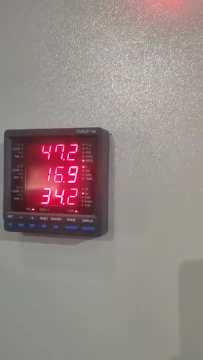 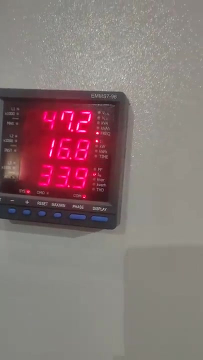 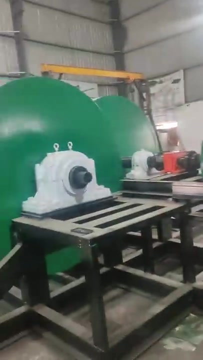 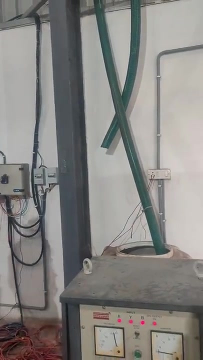 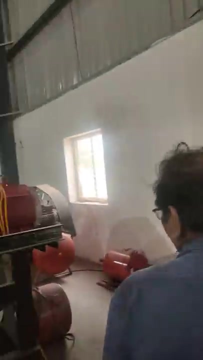 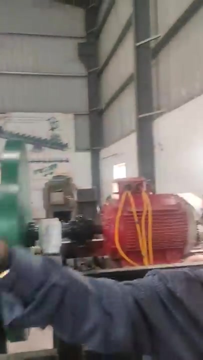 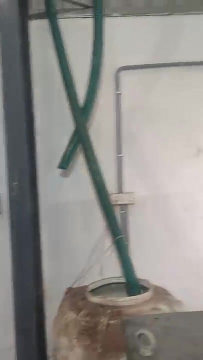 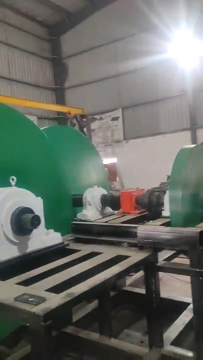 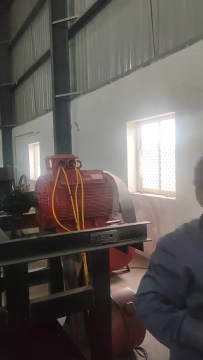 Now we will 34 am. Yeah, 165.4, Yeah, Yeah, Yeah, Yeah, Yeah, Yeah, Okay, Yeah, Yeah, Yeah. Still Resistive load. It will take a lot of time. Deceleration time is more. If the load is resistive Inductivity load, Then it will balance. 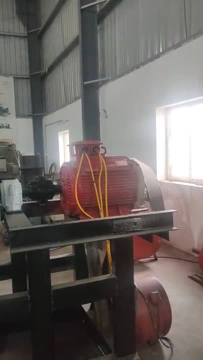 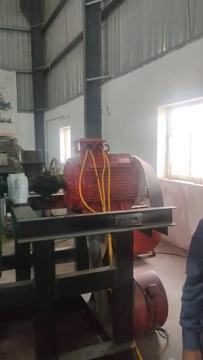 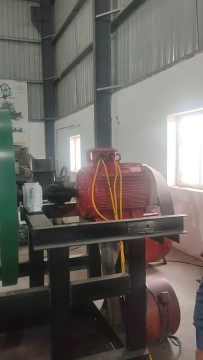 Once we increase the diameter of the flywheel And make the flywheel into Spoked flywheel, Where the energy is centered on the periphery, Will give you more energy On the outskirts of the flywheel On the heavy rim If the energy is surfaced on the outskirts of the rim.